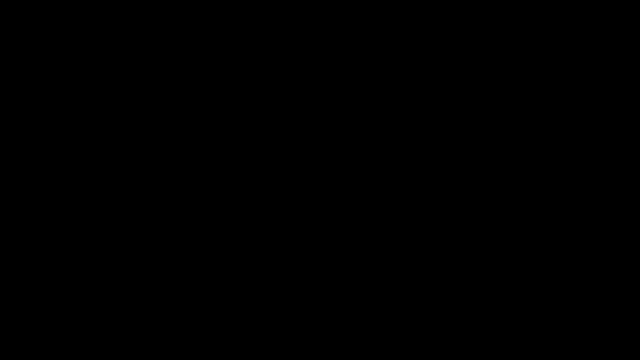 In this video, we're going to focus on solving a system of linear equations using the substitution method. So let's start with this problem. Let's say that y is equal to 2x plus 8 and y is equal to 5x minus 1.. 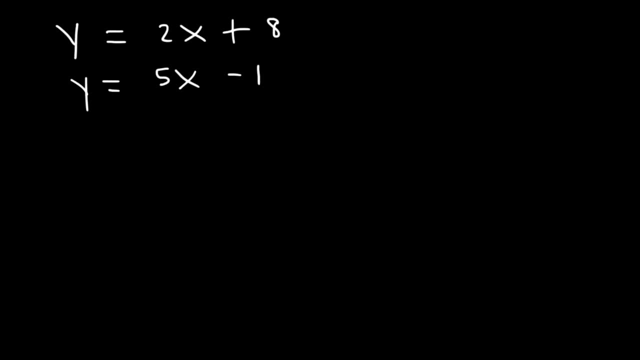 How can we find the value of x and y given these two equations? What we need to do is replace y with 5x minus 1, because they're equal to each other. So therefore, 5x minus 1 is equal to 2x plus 8.. 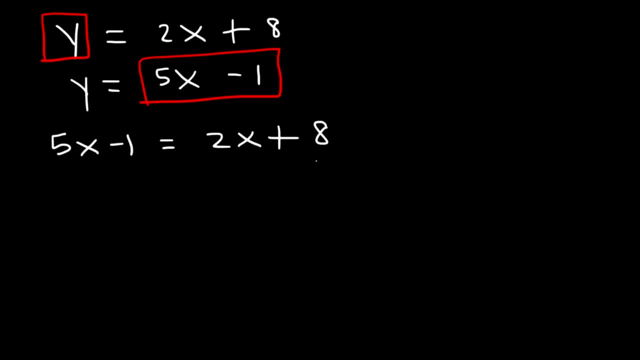 So now we have one equation with one variable, so we can go ahead and solve it. Let's add 1 to both sides. Negative 1 plus 1 is 0, so that's going to cancel. So we have: 5x is equal to 2.. 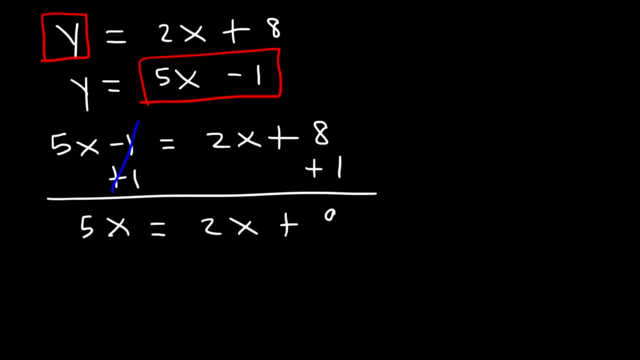 2x plus 8 plus 1, which is 9.. Our next step is to subtract both sides by 2x. 5x minus 2x is 3x, and that's equal to 9.. Now the last thing that we need to do here is divide both sides by 3.. 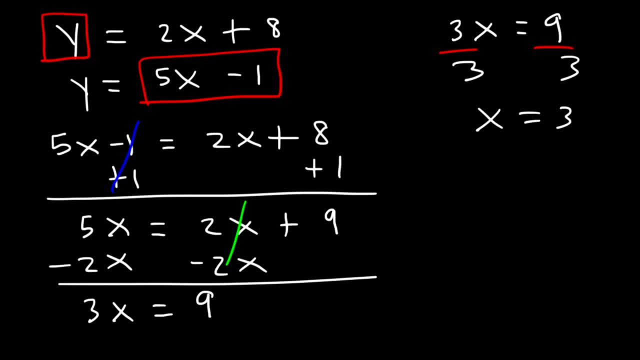 9 divided by 3 is 3, so this is the first part of the answer. x is equal to 3.. Now, now that we have this value, we can plug it into the first equation or the second, which will give you the same answer. 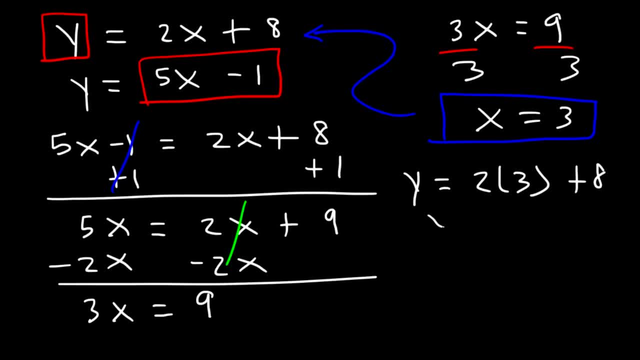 So it's going to be 2 times 3 plus 8.. 2 times 3 is 6, and 6 plus 8 is 14, so y is equal to 14.. So if you want to write your solution as an ordered pair, 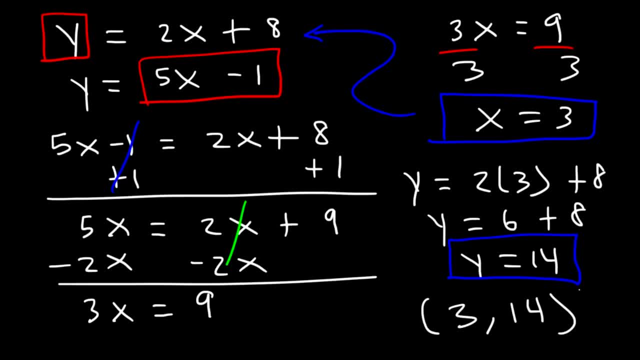 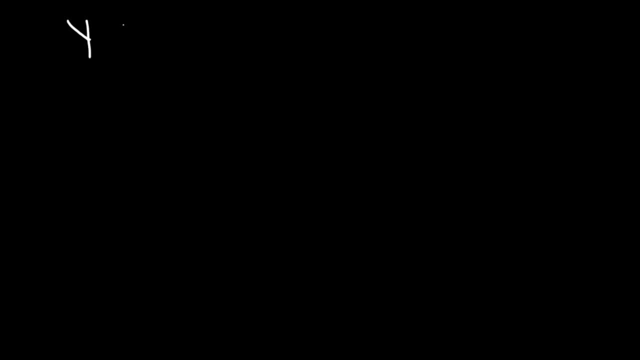 you can write like this: It's going to be 3 comma 14, and so that's the answer. Now let's work on another example. Let's say that y is equal to 2 over 3x minus 4, and also y is equal to 1 fourth x minus 3 over 2.. 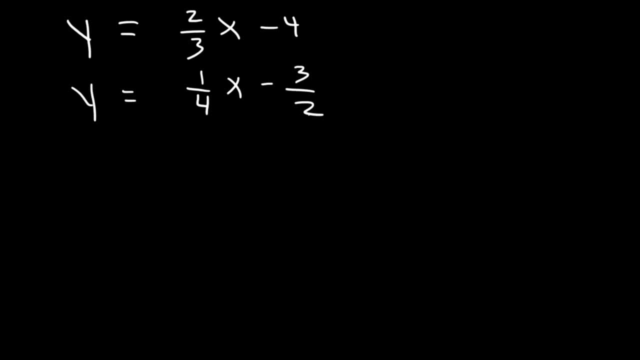 So it's very similar to the last problem, but this time we have fractions. So whenever you see two equations where y is equal to some function, you want to set these two equal to each other. It's basically the same as replacing this y with 1. fourth x minus 3 over 2.. 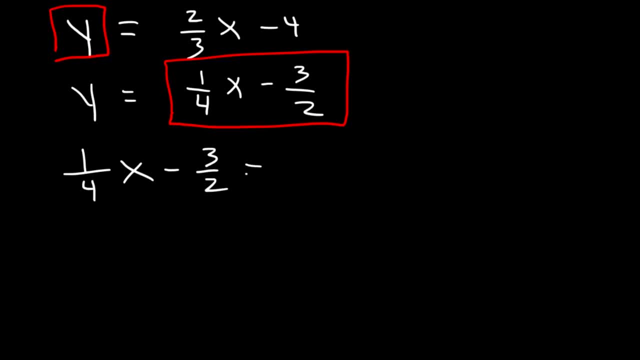 So 1 fourth x minus 3 over 2 is equal to 2 over 3x minus 4.. So what can we do in order to solve this particular equation? The best thing to do is to get rid of all the fractions. 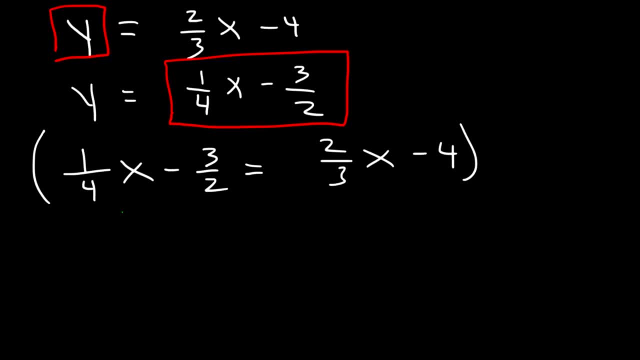 We need to find the least common multiple of the denominators 2,, 3, and 4.. What's the least common multiple between 2,, 3, and 4?? Well, we don't have to worry about 2, because multiples of 4 are the same as multiples of 2.. 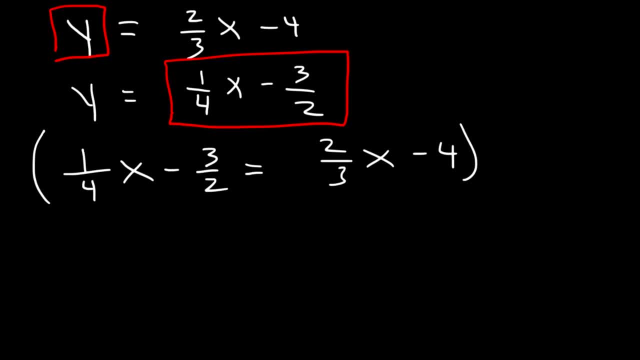 Every multiple of 4 is a multiple of 2.. So let's focus on 4 and 3.. Multiples of 4 are 4,, 8, and 12.. Multiples of 3 are 3,, 6,, 9, and 12.. 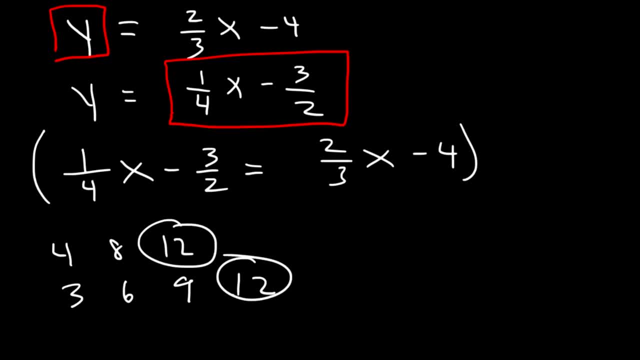 So 12 is the common multiple between 2, 3, and 4.. What do you like to do? You can divide 12 by 4, by 2, by 3, and get a whole number. So let's multiply everything by 12.. 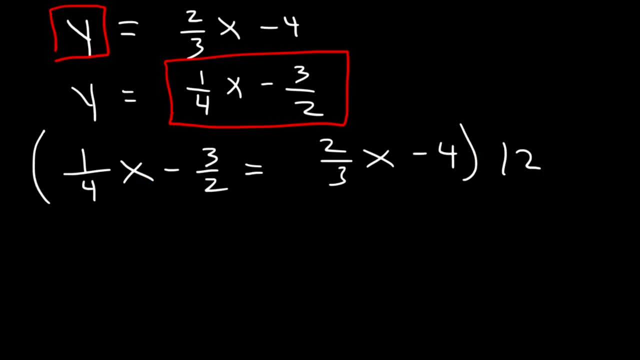 So 1 fourth x times 12.. That's basically 12 divided by 4 times x. 12 divided by 4 is 3, so that's going to give us 3x. Now what's 3 over 2 times 12?? 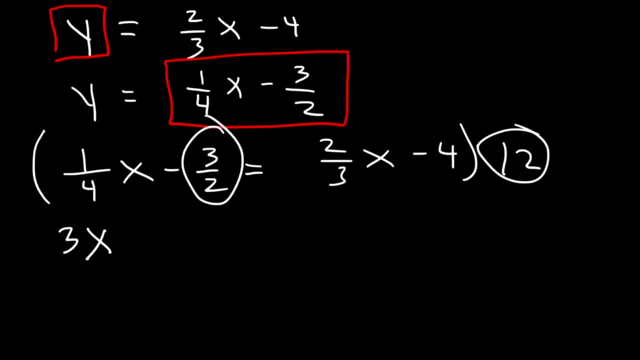 12 times 3 is 36.. 36 divided by 3 is divided by 2 is 18.. You can also do it this way: Instead of multiplying 12 by 3,, you can take 12 divided by 2,, which is 6, and then multiply it by 3, and that will give you the. 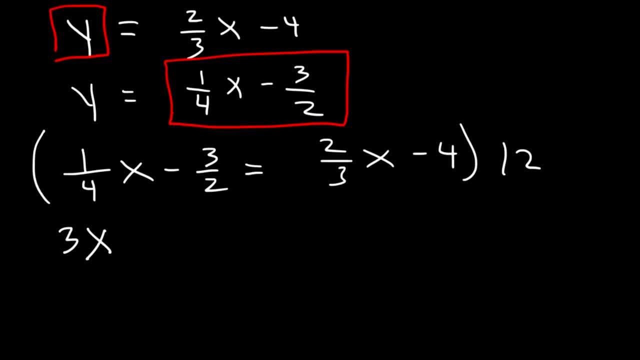 same thing, which is 18.. So what we have here is a negative 18.. 2 thirds times 12.. 12 divided by 3 is 4.. 4 times 2 is 8.. So 2 thirds of 12 is 8. And 12 times 4, that's 48.. So now, 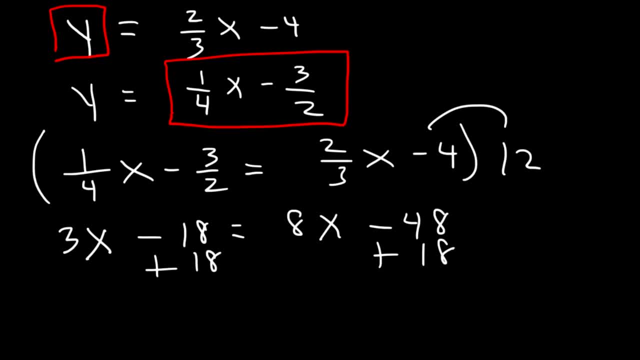 let's add 18 to both sides and simultaneously let's subtract 8x from both sides, So these will cancel: 3x minus 8x is negative, 5x Negative, 48 plus 18 is negative 30. So if we divide both sides by negative 5, we can see that x is equal. 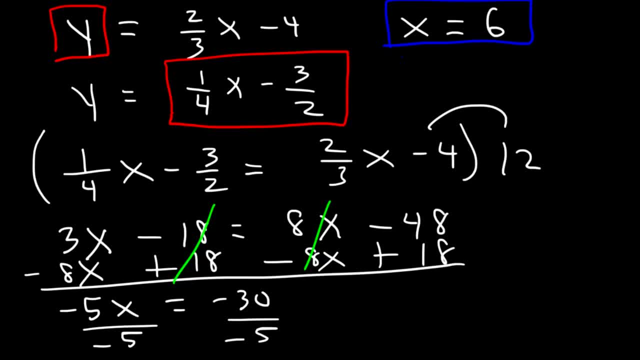 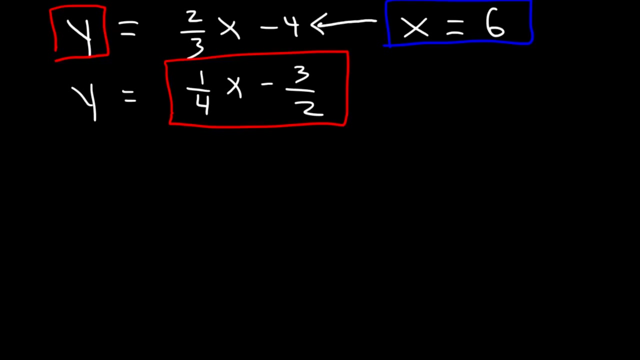 to positive 6.. So now, let's get rid of this stuff. Now all we need to do is plug in the 6 into the first or the second equation, But let's use the first one. So let's replace x with 6.. So what's 2 thirds of 6?? 2 times 6 is 12, divided by 3, and that's 4.. And 4. 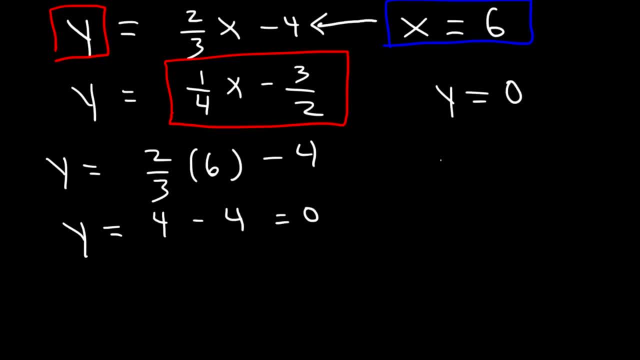 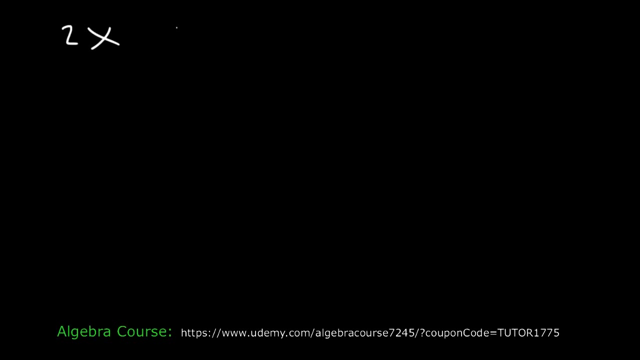 minus 4 is 0. So y is equal to 0. So in terms of x comma y, as an ordered pair, it's going to be 6 comma 0. So that is the solution for this example. Here's another problem. Let's say that 2x plus 5y is equal to 19. And also that y is 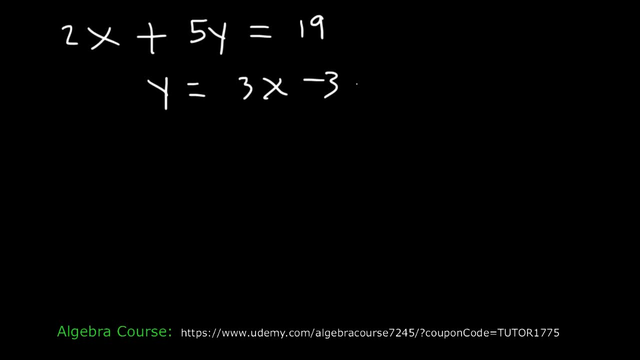 equal to 3x minus 3.. So the setup is a little different, But feel free to pause the video and try this example. Go ahead and find the value of x and y. So because we have y by itself in the second equation, we can replace y in the first equation with 3x minus 3.. So 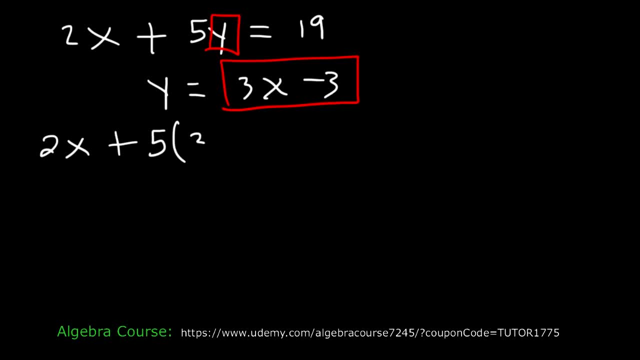 thus we'll have this expression: 2x plus 5 times 3x minus 3 is equal to 19.. So all we get to do is take this and insert it into or replace y with that expression. So now let's distribute the 5. 5 times 3x is 15x and 5 times negative 3 is negative 15.. So 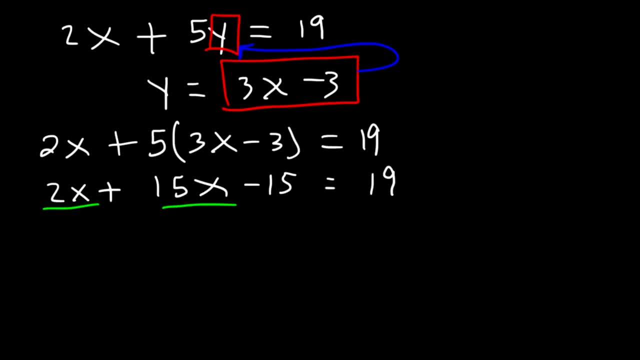 now let's combine like terms 2x plus 15x and that adds up to 17x. In our next step we can add 15 to both sides, So we have: 17x is equal to 19 plus 15, which. 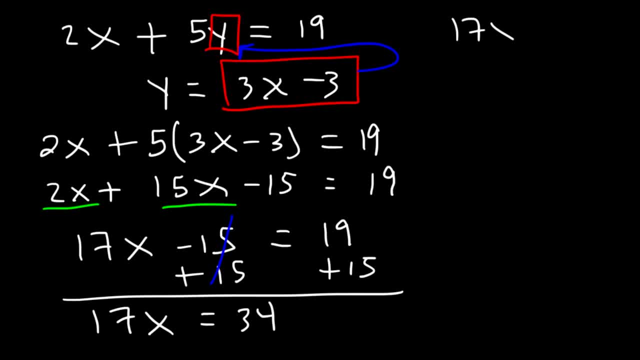 is about 34.. Next we need to divide both sides by 17.. 17 goes into 34 two times. Therefore, x is equal to 2.. Now, once we have x, let's plug it into this equation, because we already have y by itself. 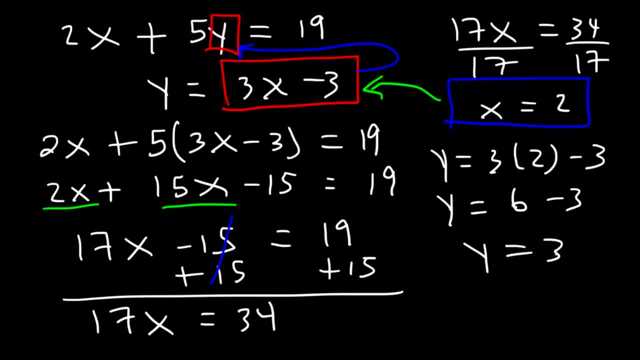 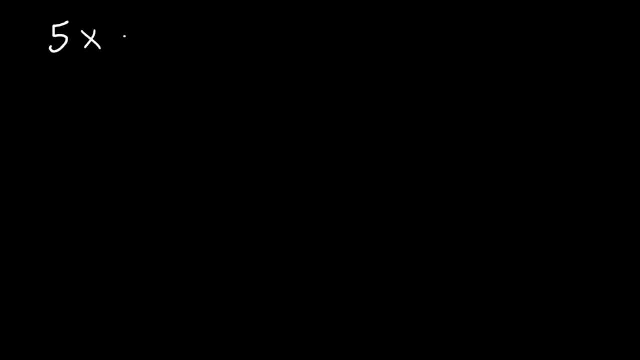 3 times 2 is 6.. 6 minus 3 is 3.. So y is equal to 3.. So our answer as an ordered pair is 2 comma 3.. And so this is the solution. Here's another similar problem. Let's say that 5x. 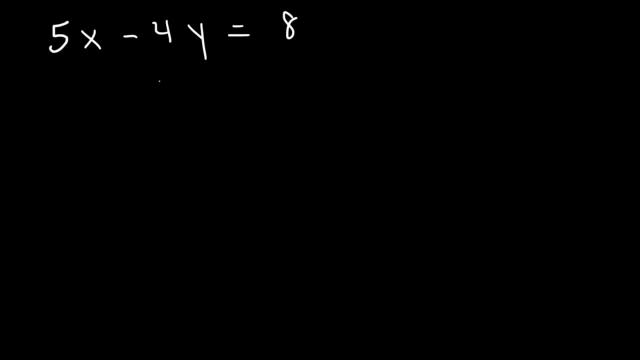 minus 4y 7 is equal to 8.. And also that y is halved down by 1.. 1 half x plus 1.. Go ahead and take a while to work on that problem. Just like before were going to replace y with halved x plus 1.. So let's take this. 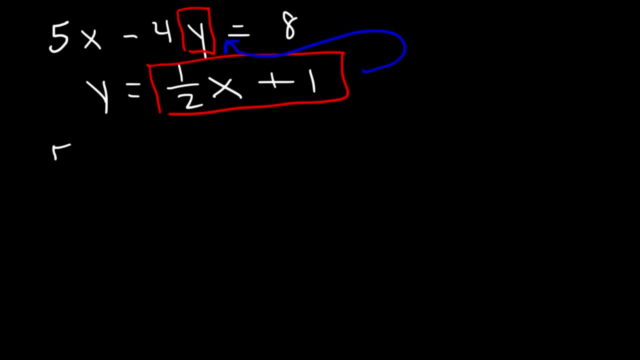 and put it into our first equation. So we're going to have 5x minus 4 times 1, half x plus 1. And that's equal to 8.. So now let's distribute the 4. 4 times 1 half is basically 2.. So we're going to have negative 2x, Negative 4 times 1, that's negative 4.. And now we could combine like terms: 5x minus 2x is 3x. 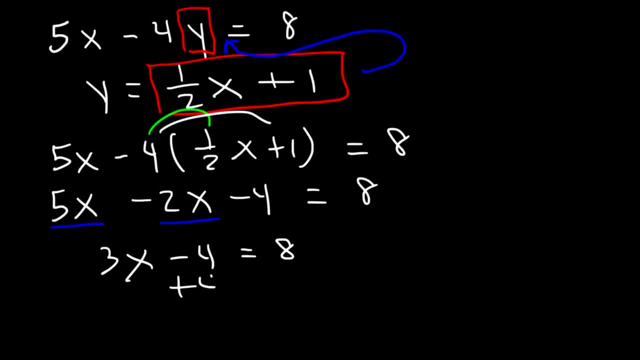 And in the next step we can add 4 to both sides. 8 plus 4 is 12.. And 12 divided by 3 is equal to 4.. So now that we have x, let's plug it into the second equation to get y. 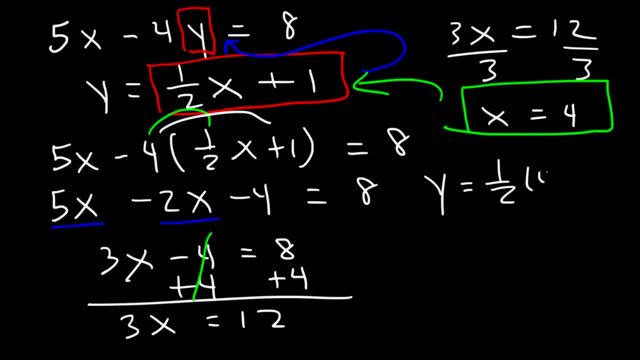 So y is going to be 1 half Times 4 plus 1.. Half of 4 is 2., And 2 plus 1 is 3.. So y is equal to 3.. So our solution is 3 comma actually. no, it's 4 comma, 3.. 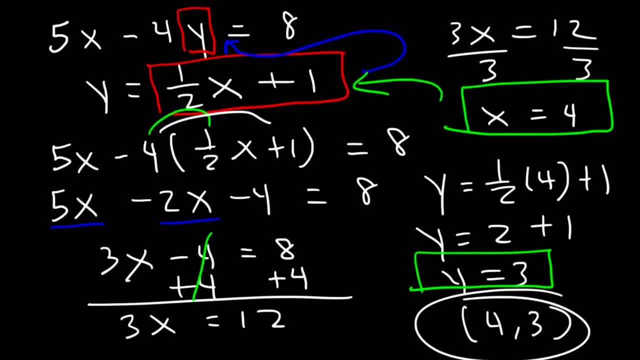 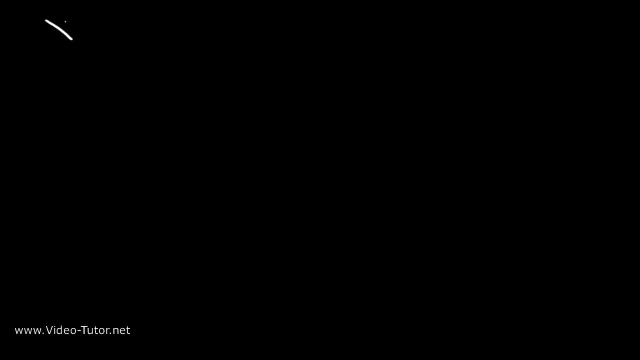 Rather than 3 comma, 4.. x is 4 and y is 3.. So that's it. Let's try an example with 3 equations and 3 variables. So let's say that x plus y plus z Is equal to 6..